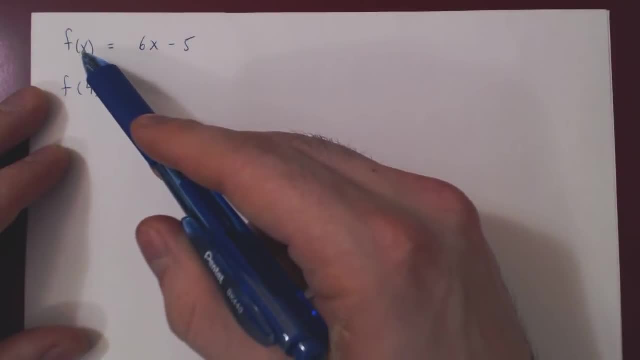 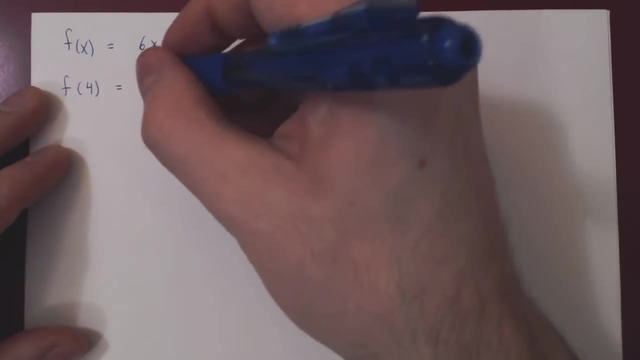 We are making a substitution. We are replacing the argument x in the expression by the value 4.. So we replace everywhere x by 4.. So we get 6 times 4 minus 5, which gives us 24. Minus 5.. 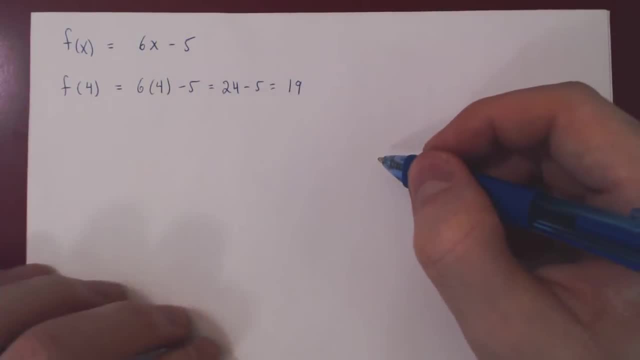 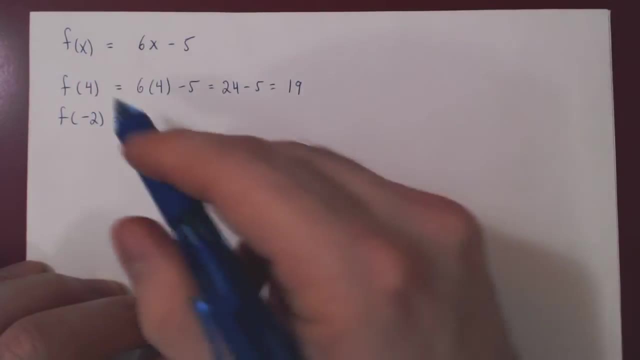 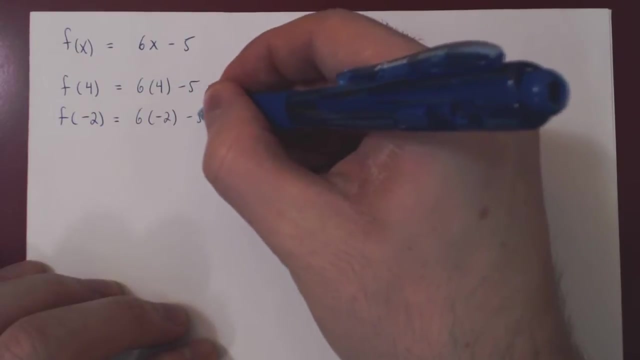 Minus 5,, which gives us 19.. And that's f of 4.. We could calculate f of, say, negative 2.. Same thing. now we are replacing x by the value negative 2. So we'll get 6 times negative 2, negative 5,, which gives us negative 12.. 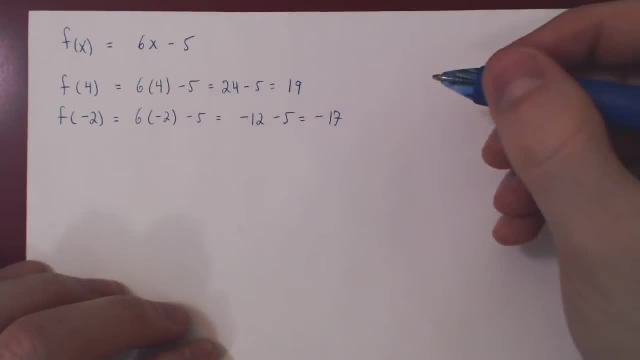 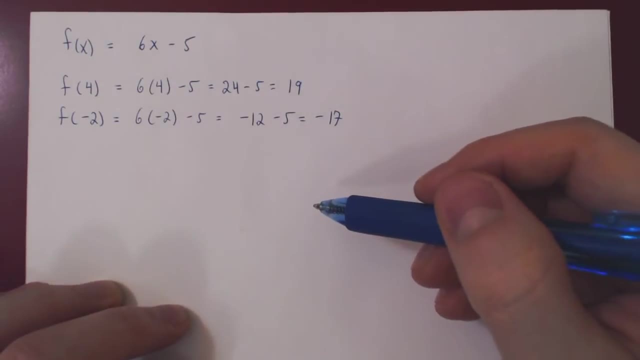 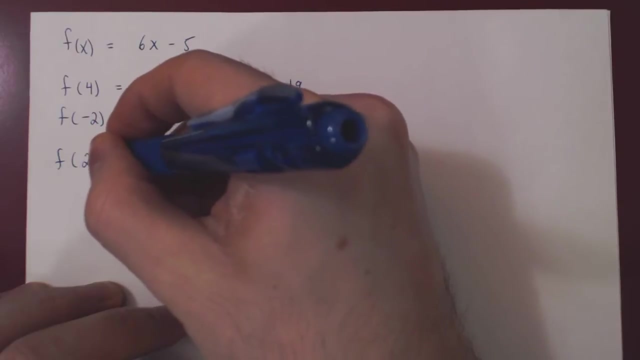 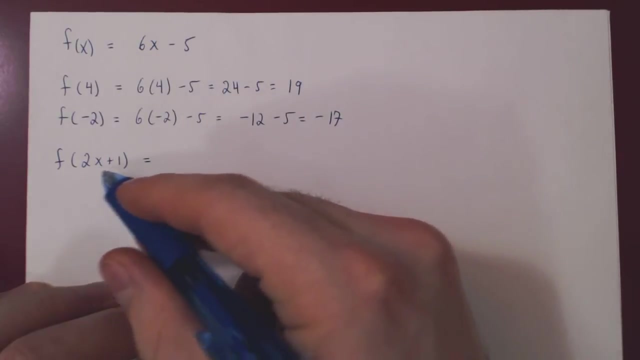 Negative 5, which gives us negative 17.. We can also replace x by not only real numbers, but by other variables. So for example, we could replace x by, say, 2x plus 1.. So now we are making a more interesting substitution, right. 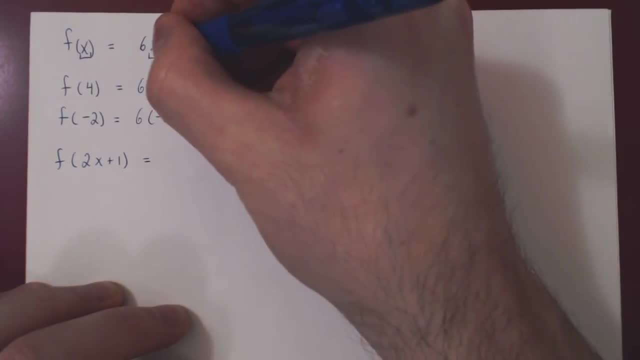 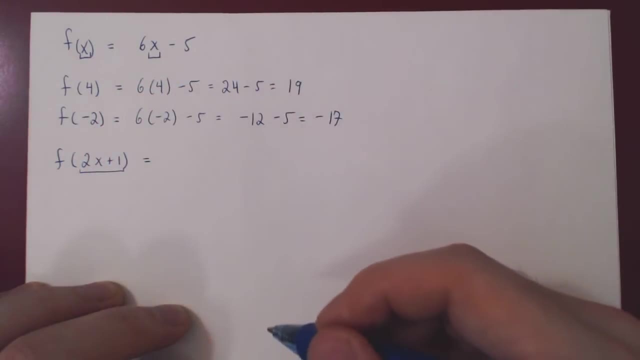 If you go back, f of x equals 6 times x minus 5.. But now we are replacing x by the new variable 2x plus 1.. So let's replace every variable. So let's replace every variable- We're in the expression where there's an x by the new argument 2x plus 1.. 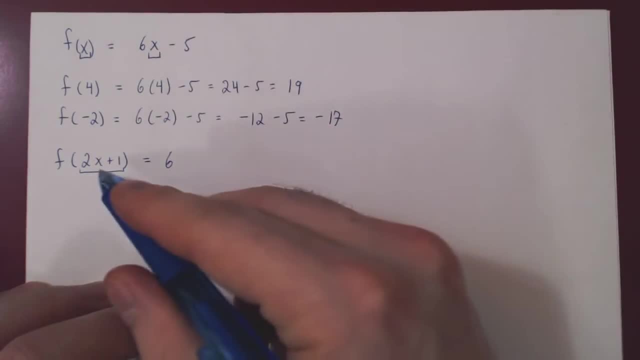 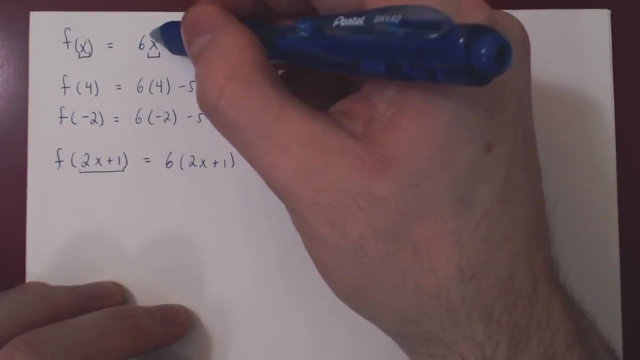 So we get 6 times no longer x, but 2x plus 1.. Be careful to have parentheses here, as all of the argument, which is now 2x plus 1, is being multiplied by 6.. There is no x with the 5, and that's just negative 5.. 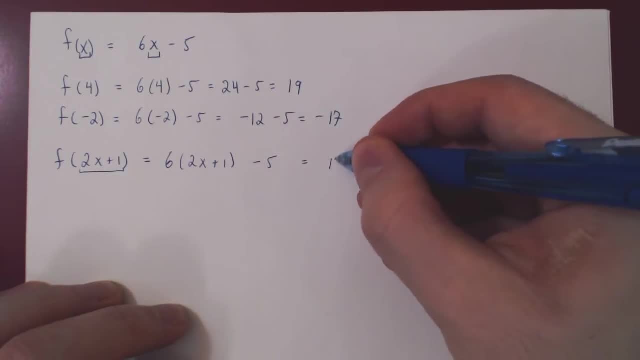 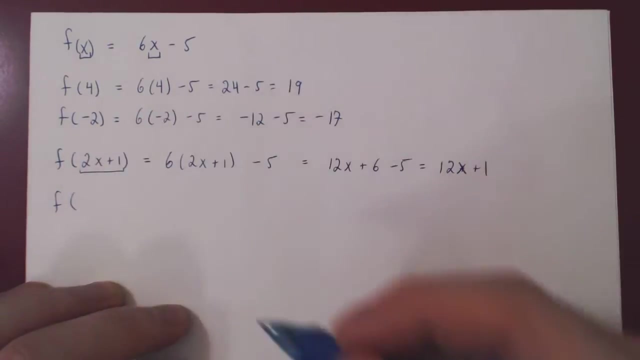 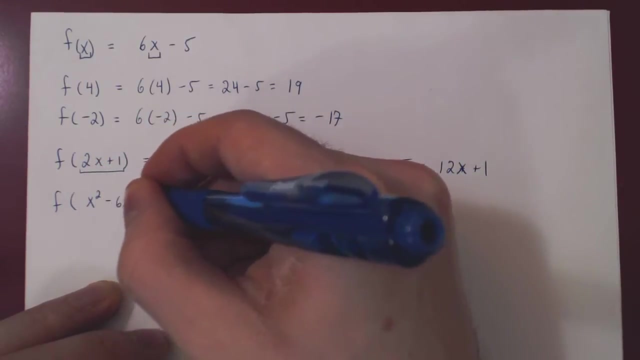 And now we can simplify: Multiply out, we'll get 12.. x plus 6 minus 5,, which gives us 12x plus 1.. We could replace x by, say, a quadratic polynomial: x squared minus 6x plus 4.. 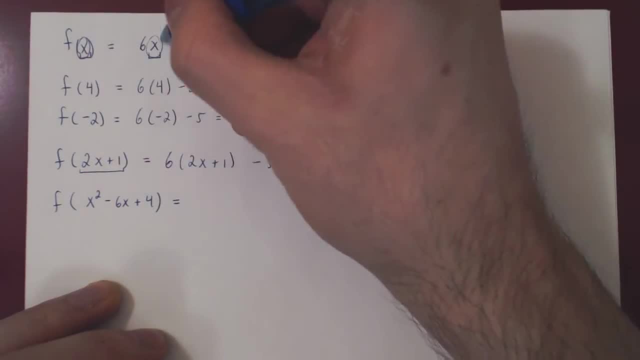 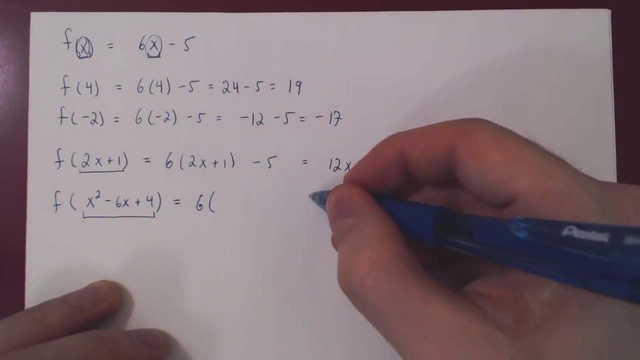 Once again we are replacing x everywhere in the expression, but the new argument, which is x squared, is negative 4. So we get 6 times the new argument: x squared minus 6x plus 4, minus 5.. 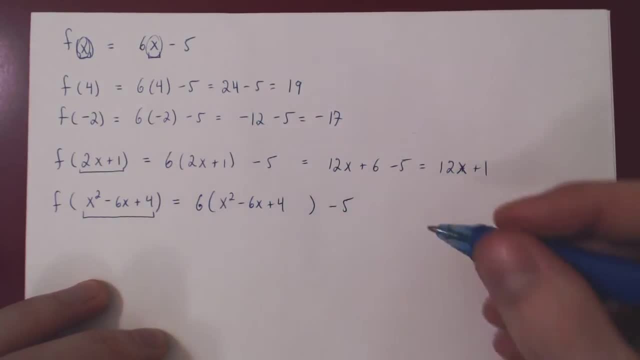 There is no x, so it stays negative 5. We could multiply out 6x squared minus 36x, plus 6 times 4, 24, minus 5,, positive 19.. Let's make one more substitution. 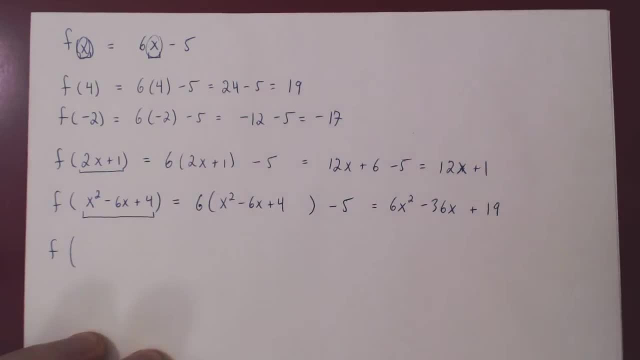 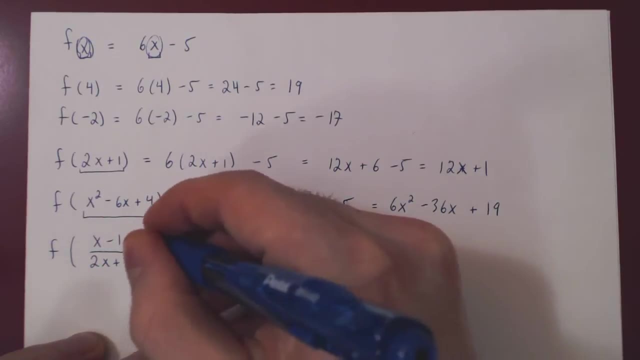 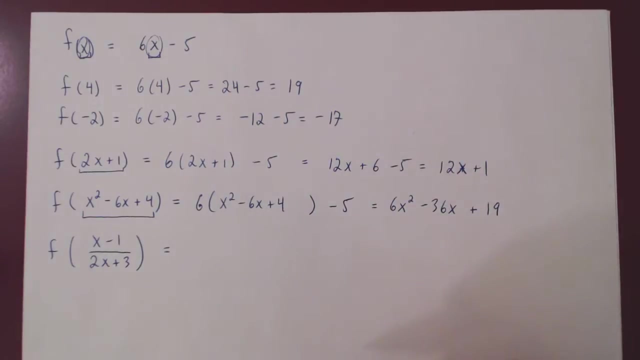 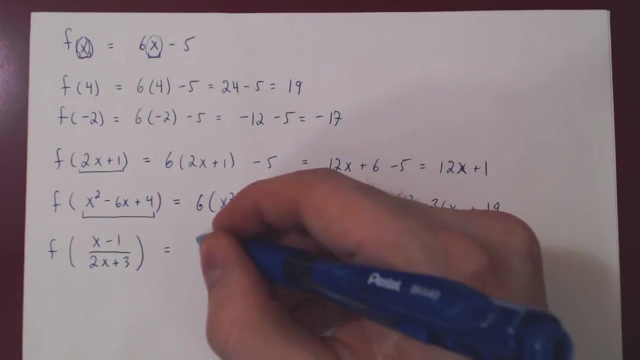 We could replace the argument x by, say, a rational function. What about x minus 1 over 2x plus 3?? So everywhere we replace the old argument, that was x, by the new argument, which is this rational function, So 6 times the new argument. 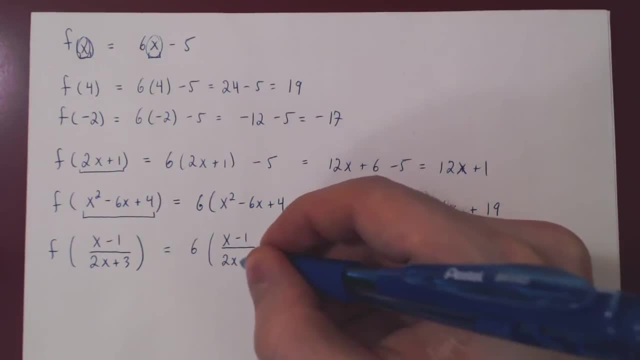 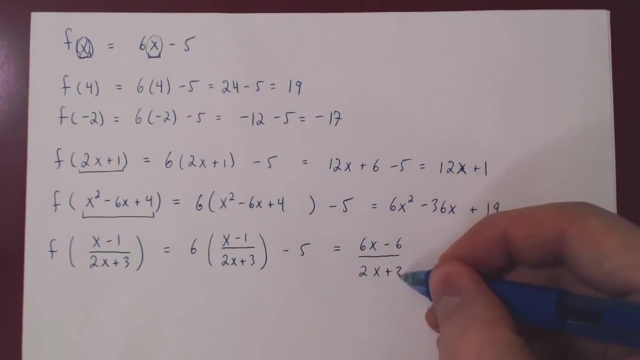 So 6 times the new argument minus 5,. we could combine as a single fraction, so 6x minus 6, over, 2x plus 3, minus, and to have a common denominator we'll multiply top and bottom by 2x plus 3.. 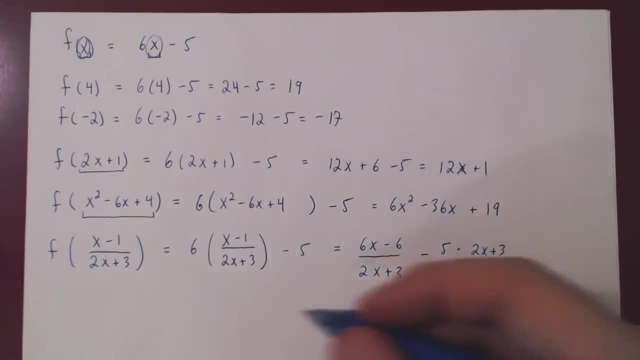 So what will that give us? 6x minus 6, over 2x plus 3, minus. we can multiply now the numerator by 5, which will give us 10x plus 15, over 2x plus 3.. 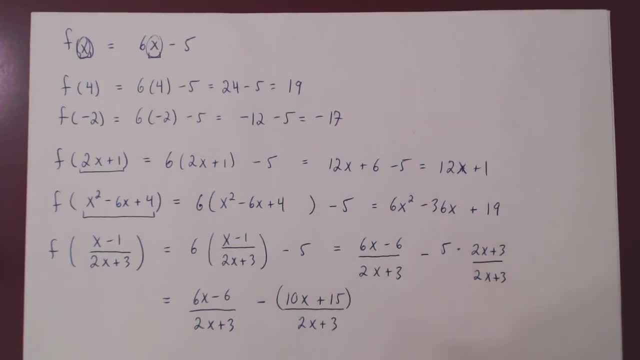 And be careful. the negative is applied to the entire numerator And now, as both fractions are under a common denominator, we can combine, So we'll get 6x minus 10x, which is negative, 4x, negative, 6, negative 15, negative 21,, over 2x plus 3.. 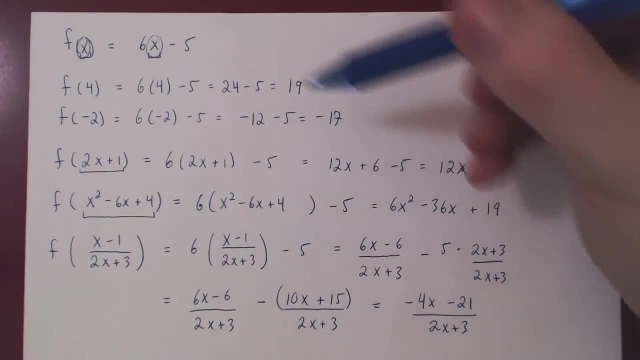 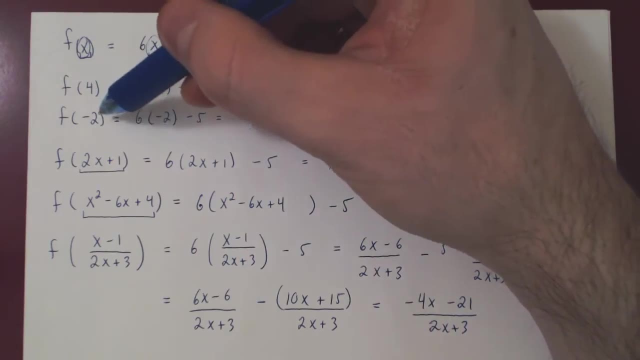 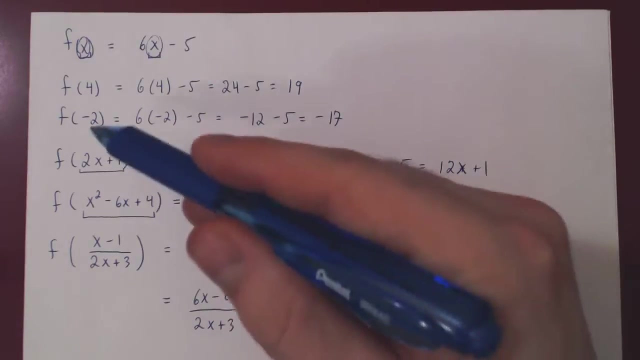 So there you go. So the idea is: If you're given a function, because x is a variable, you can replace the argument x by anything you want, either by a real value or by any other given variable. We could also replace x by not only one, but several other variables. 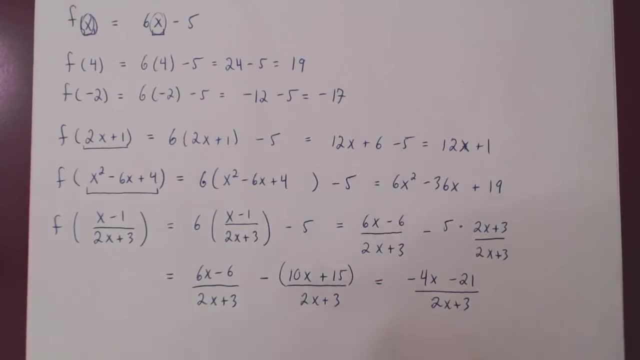 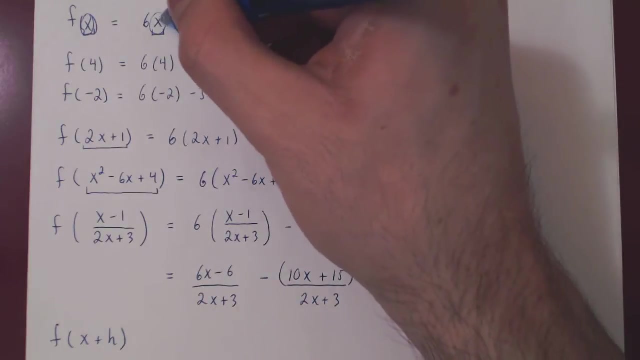 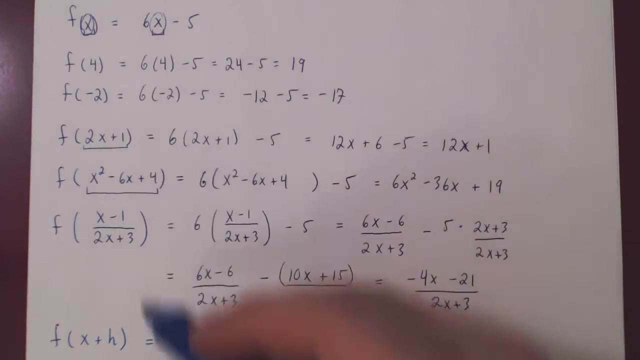 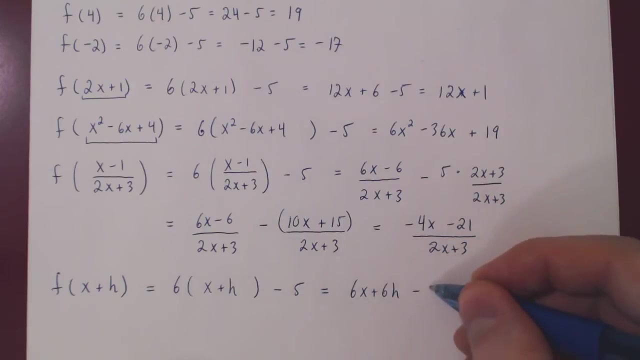 Let's just go with one other example. So suppose we replace x by a sum of two variables, say x plus h. So here x is a variable, h is a different variable. and now again we replace 6 times no longer x, because we have replaced x by x plus h. so 6 times x plus h minus 5, stays negative 5, and so we get 6x plus 6h minus 5.. 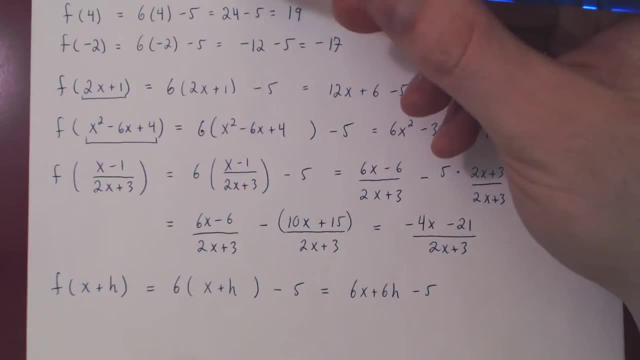 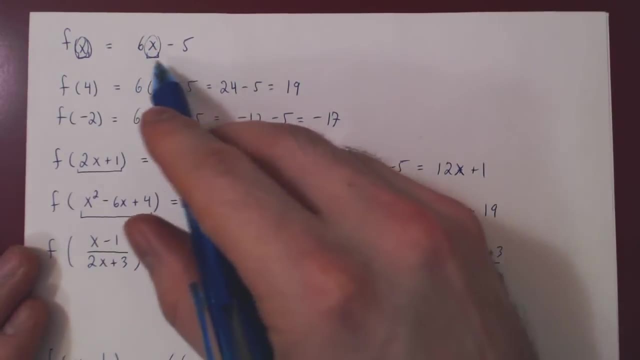 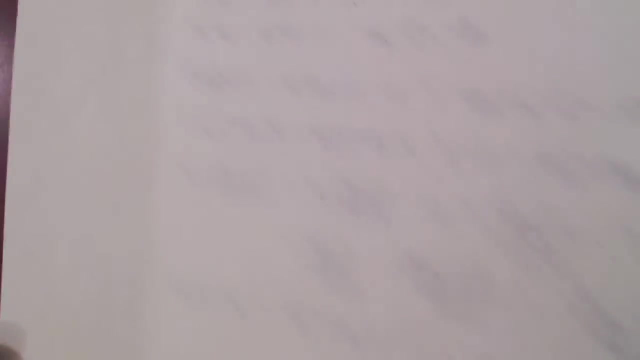 And that's it. Let's do a few more examples now with a different function. This was rather a simple function. 6x minus 5 was a linear function. Let's use, say, a quadratic function, And then we'll use a rational function. 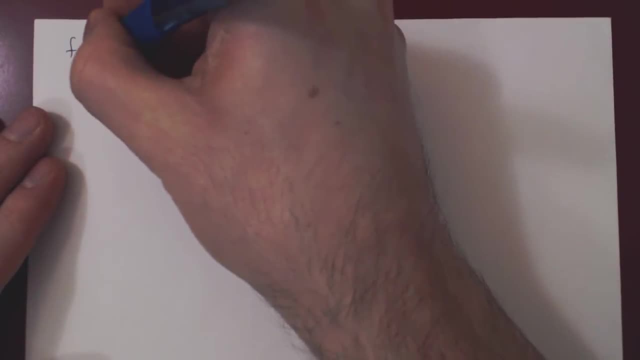 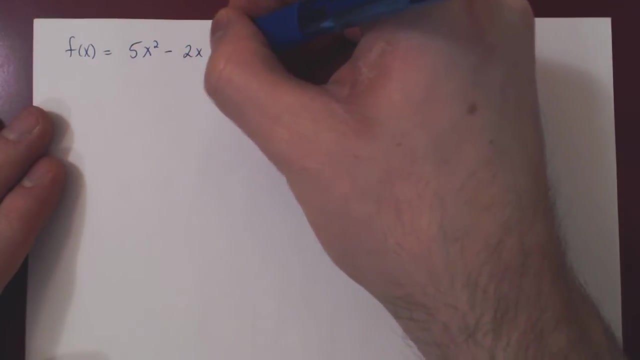 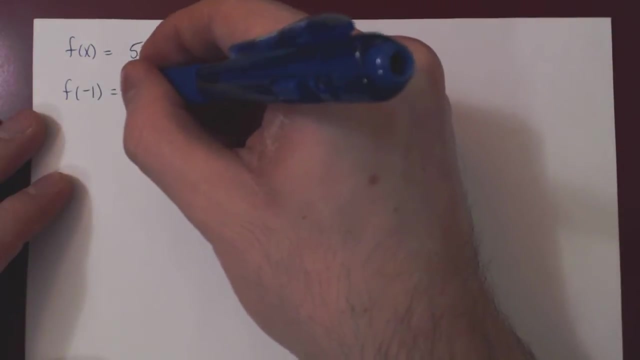 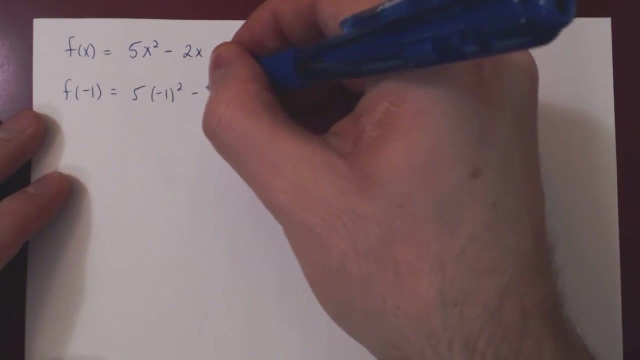 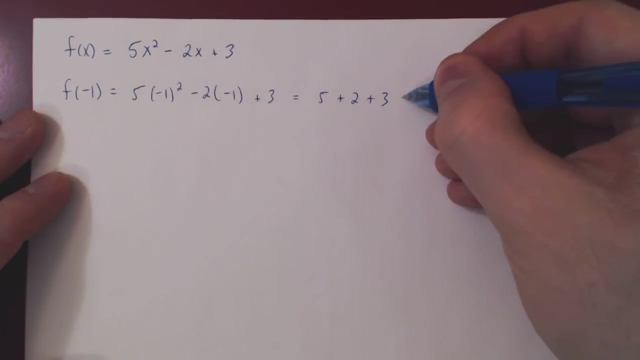 So what if we take f of x To be 5x squared minus 2x plus 3.. We could take f of negative 1, which would be 5, and now we are replacing x everywhere by negative 1.. So 5 times negative 1 squared minus 2 times negative 1 plus 3, which gives us 5 plus 2 plus 3,, which gives us 10x. 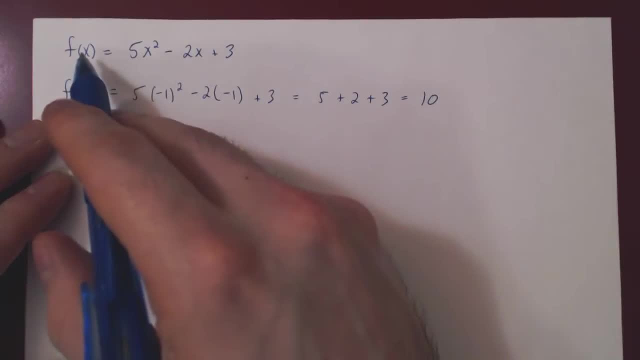 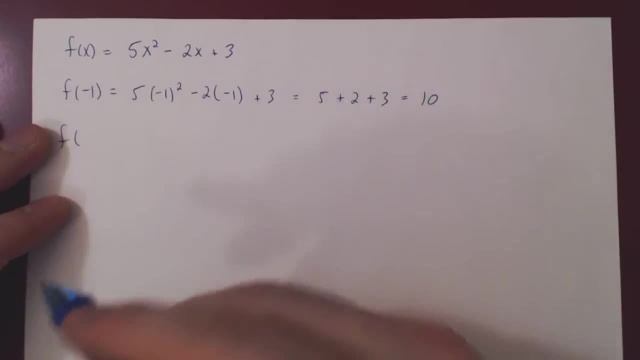 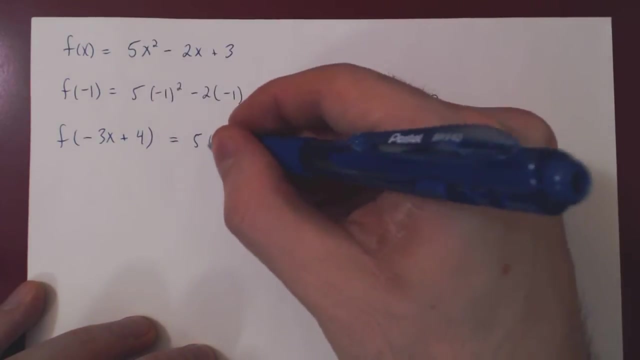 well, let's replace now x by a linear polynomial. so say: f of x will now take f of minus 3x plus 4. so we are replacing everywhere in the expression the old argument, that was x, by the new argument, which is negative, 3x plus 4. so we get 5 times no longer x, but negative 3x plus 4 squared. 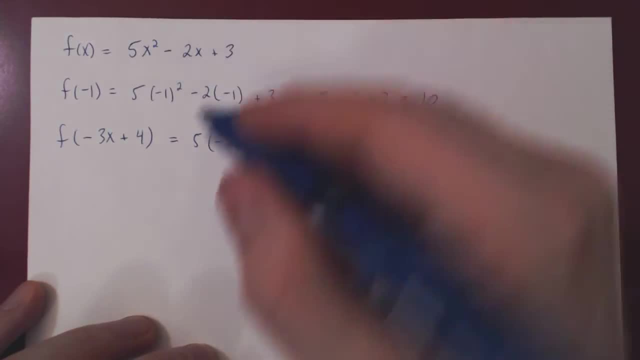 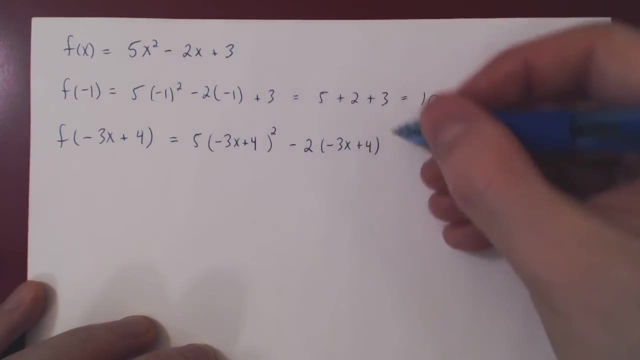 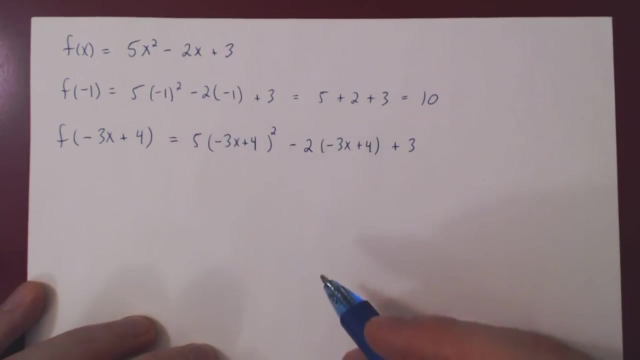 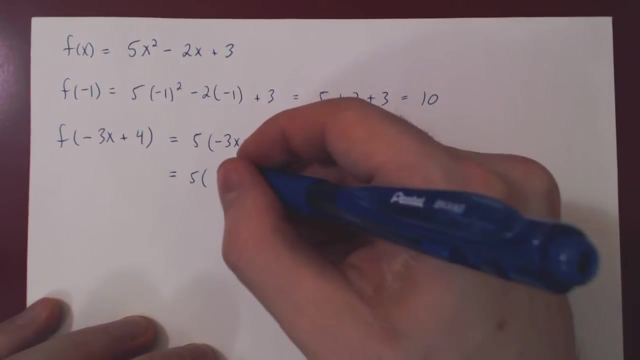 minus 2 times no longer x, but negative 3x plus 4 plus 3. there's no x, which stays plus 3. and now we can simplify, we could square this and then we regroup similar powers of x, so we'll have 5 times. if you square this, you'll get 9x squared. 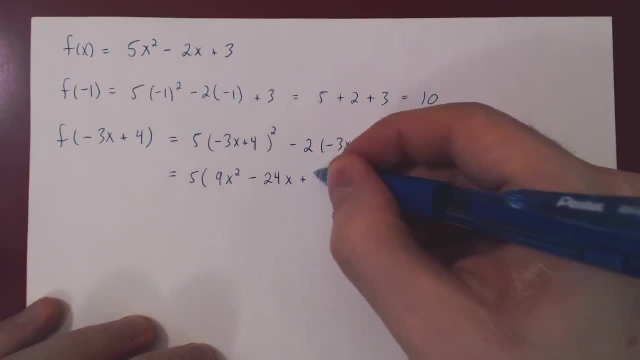 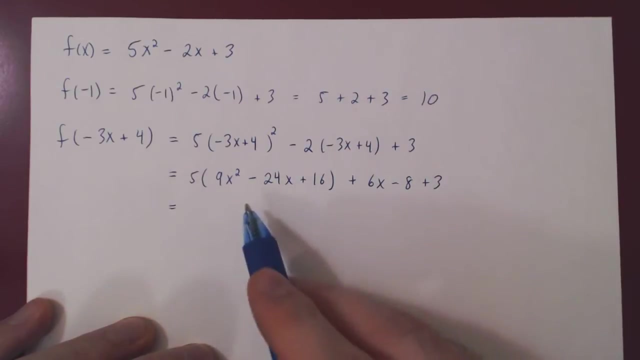 minus 24x plus 16. multiply this one out positive, 6x minus 8 plus 3, and now we can multiply through by 5 and then regroup. at the same time there's a single quadratic term: 9x squared times 5 is 45 x squared minutes. 4x squared times 5 is 45 x squared 5 times 24. well, 5 times. 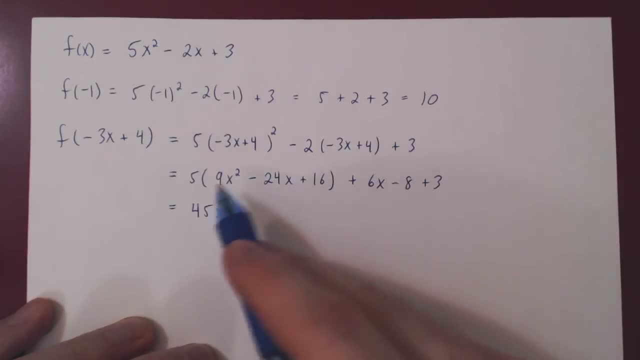 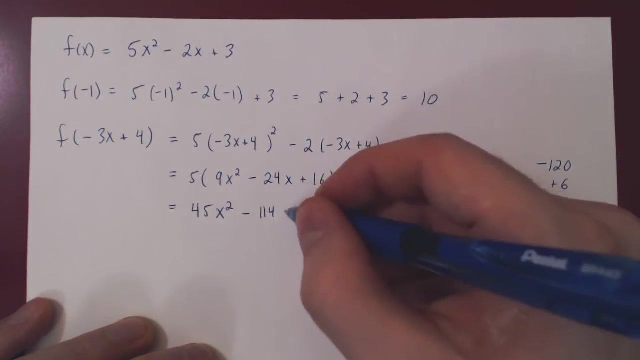 20 is 100, 5 times 4 is 20 ». so there's 120, but it's negative 120 plus 6 x. this will give us negative 114x 1012 е, 90 x 100 e 120 x 6 x. 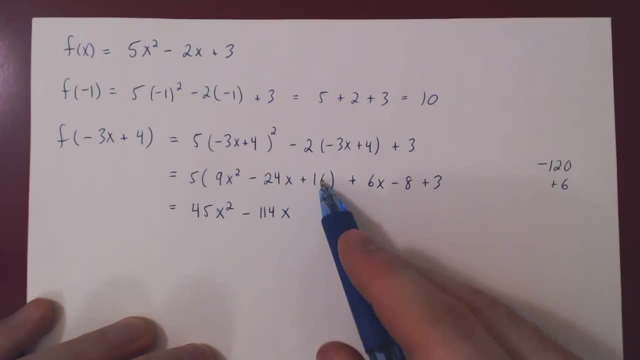 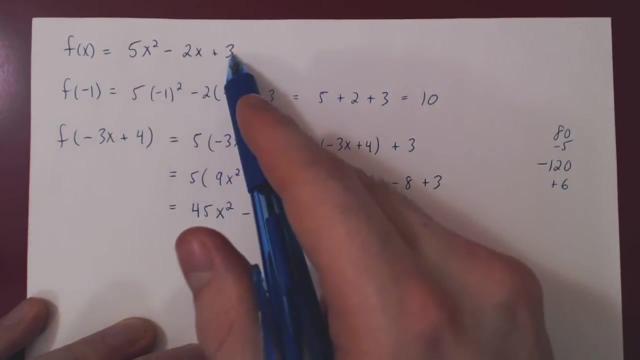 40 e terms. Well, 5 times 16 is 80.. Minus 8 plus 3 is minus 5.. This will give us positive 75.. And there you have it. If f of x is 5x squared minus 2x plus 3, replacing x in the expression, 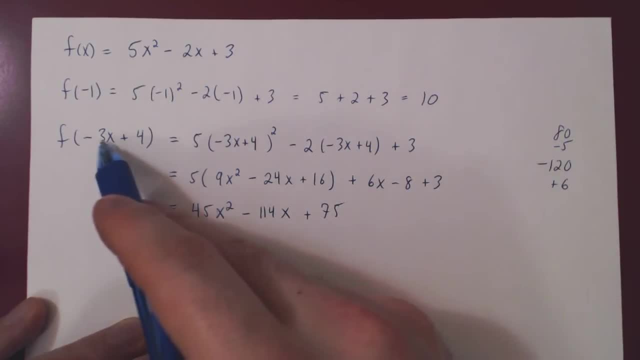 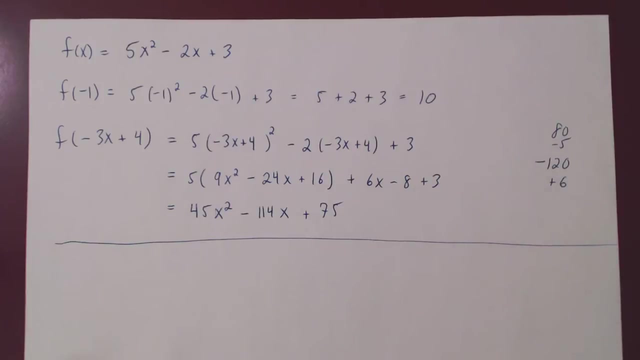 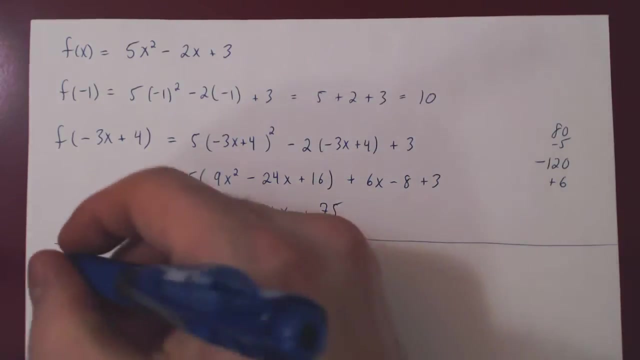 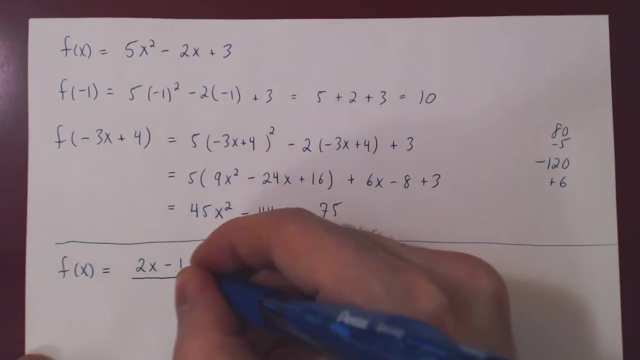 by negative 3x plus 4 gives us that f of negative 3x plus 4 is 45x squared minus 114x plus 75.. Let's do one more example now where the function is a rational function. So suppose we take f of x to be 2x minus 1 over 3 minus x. 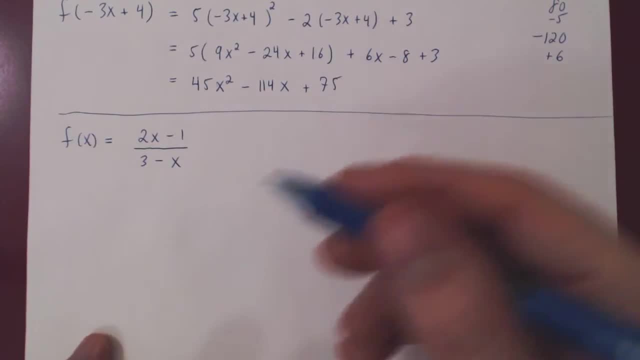 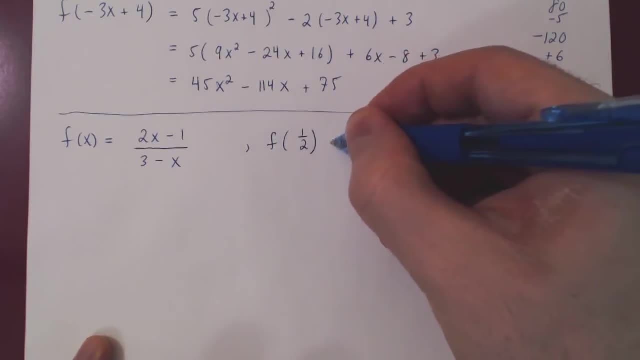 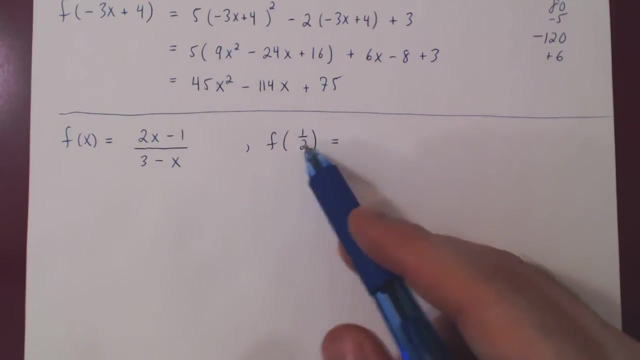 So we could evaluate f at, say, a real number. We could take f of 1 half. So now we are replacing in the expression the variable x by the real value of 1 half Here, where where there is an x we have to replace it by 1 half. 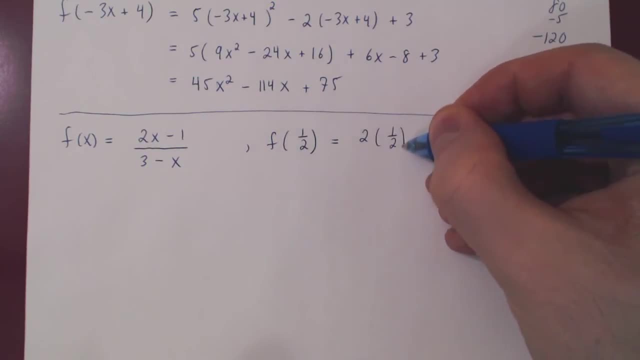 So we have 2 times 1 half minus 1 over 3 minus 1 half. But if you look on the numerator, 2 times 1 half is 1 minus 1, is 0 over 3 minus 1 half. 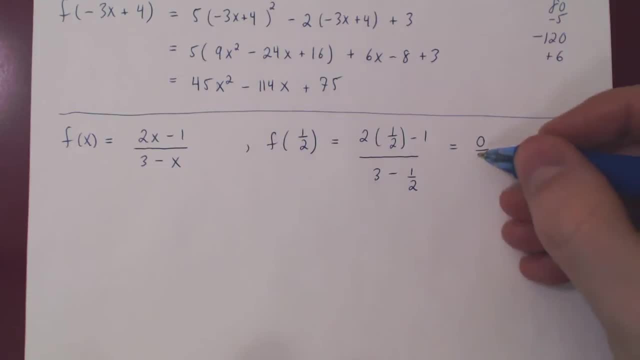 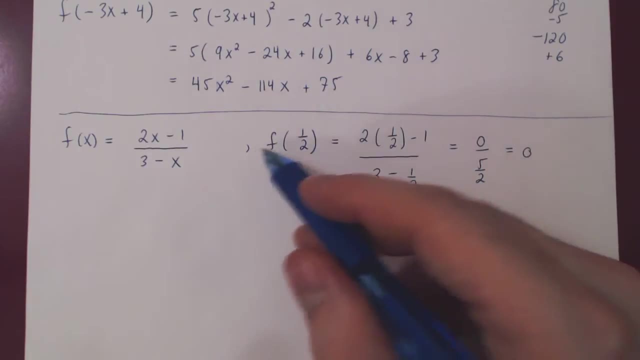 Well, 3 is 6 over 2, minus 1 half, 5 over 2.. But 0 over a constant, It's simply 0. And so we get that f of 1 half is 0.. Let's look at, say, f of 3 quarters. 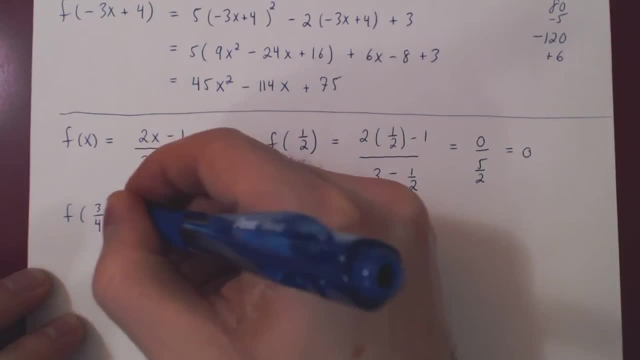 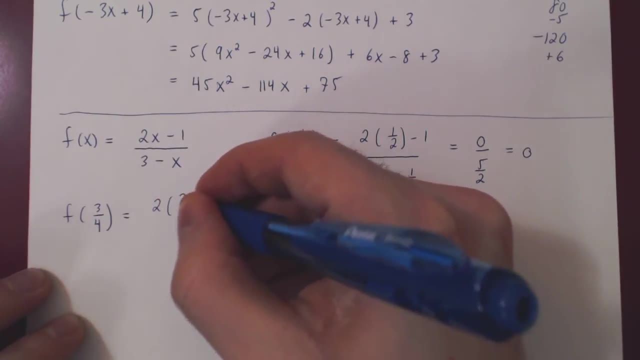 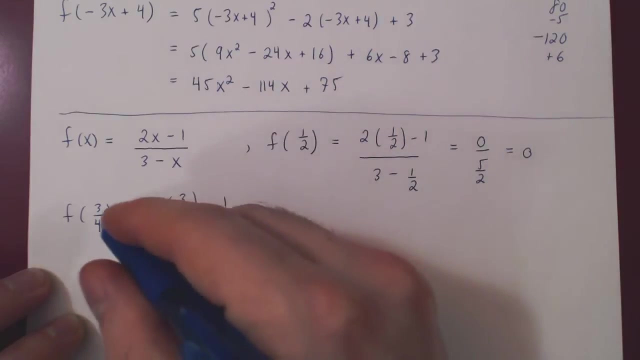 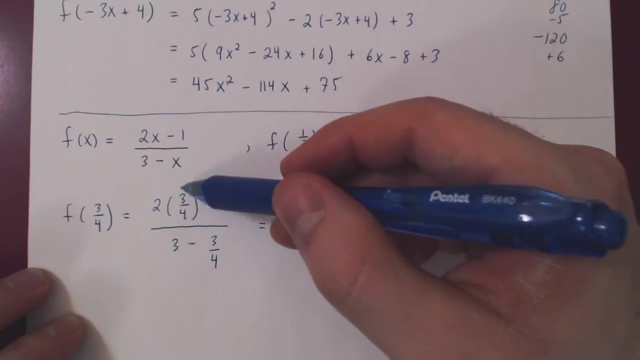 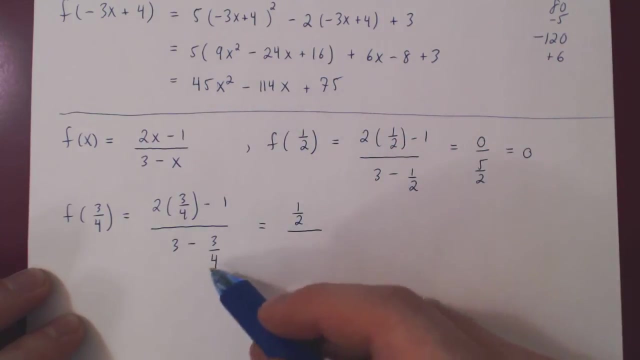 This may be a bit more interesting Now, replacing x everywhere in the argument by 3 quarters. So we get 2 times 3 quarters, minus 1 over 3, minus no longer x, but 3 quarters. Well, let's see: 2 over 4 is 1 half, 3 half minus 1 is 1 half divided by well, 3, if we put this over 4, it will be 12 over 4, so we have 1 half divided by 12 minus 3, 9, so 9 quarters. 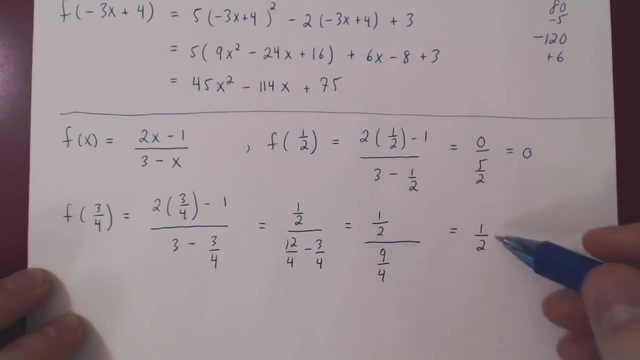 Well, we are dividing 1 half by 9 quarters if we divide by 4.. Well, we are dividing 1 half by 9 quarters if we divide by 4.. So we have a fraction. you multiply by the reciprocal, so 4 over 9.. 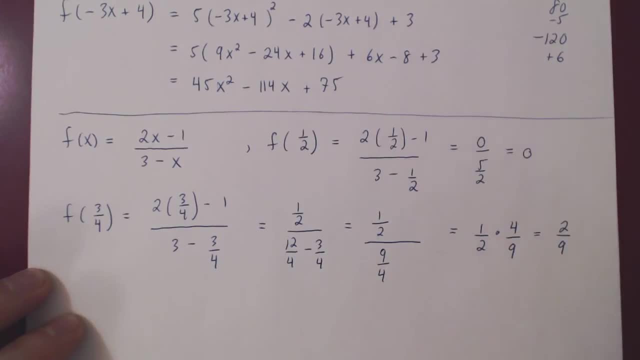 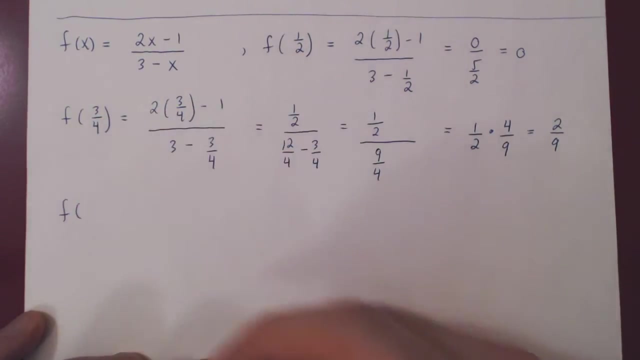 But 4 over 2 is 2, and so we are left with 2 over 9.. And so f of 3 quarters is 2 over 9.. Let's do two more substitutions. Let's look at f of, say, 5x minus 8.. 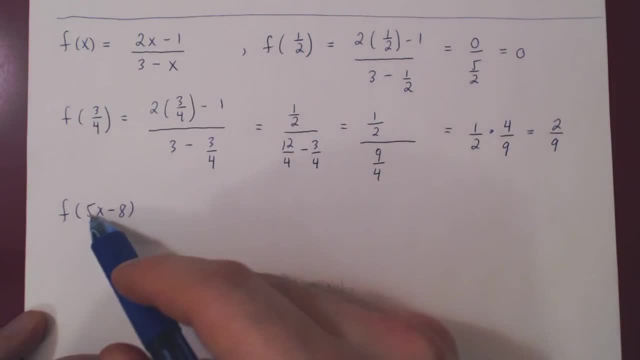 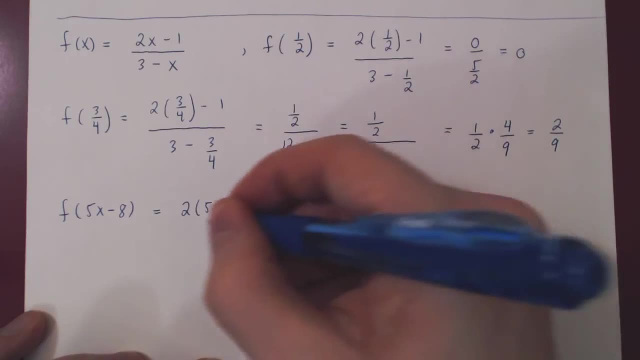 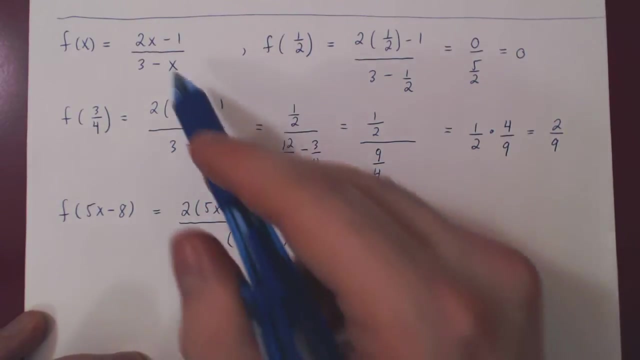 Now replacing x, replacing x everywhere in the expression- by 5x minus 8. so we get two times 5x minus 8 minus 1 over 3 minus, and here be careful to open your parentheses, because all of x has been negated. 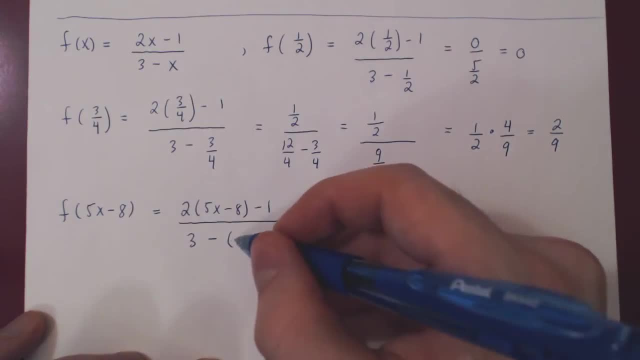 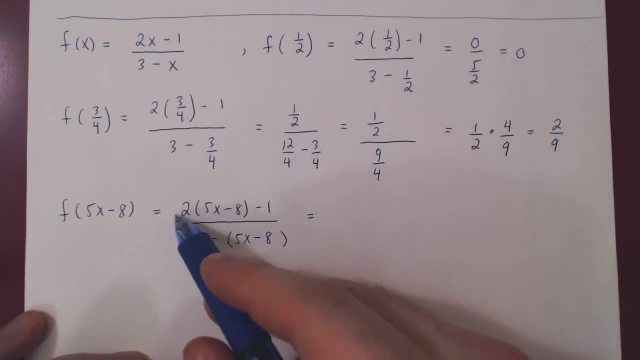 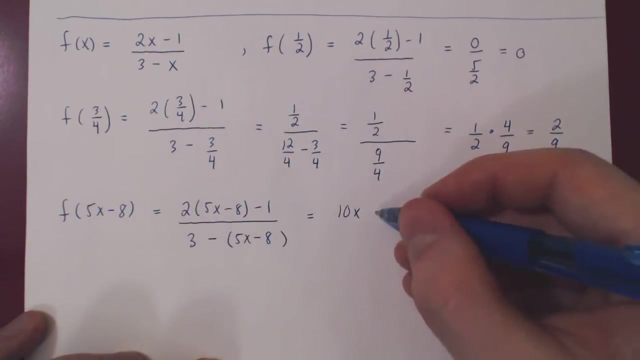 and so you have to negate all of the new variable, which is 5x minus 8. we can simplify a little bit: multiply across by 2 and subtract the 1, 2 times 5x. 10x minus 16 minus 1, minus 17 over negative 5x. but negative negative 8 is plus 8 plus 3 is 11. 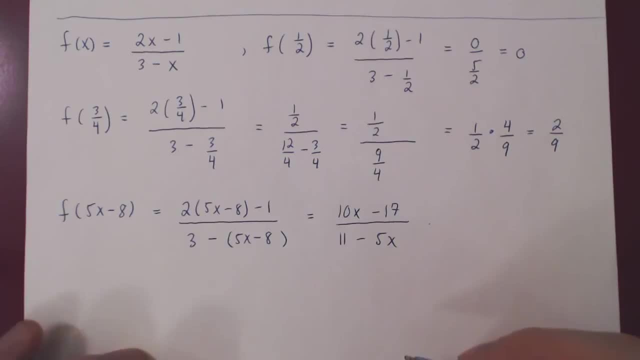 minus 5x. there you have it. now let's do one last substitution. let's replace a negative negative 8 plus 8 plus 3 plus 11 and we have a negative, negative negative 8 plus 3 plus negative negative 8 plus 3 plus 11 minus 5x. now let's do one last substitution. let's replace a 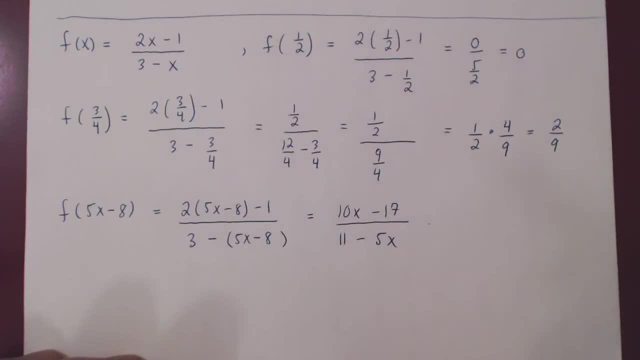 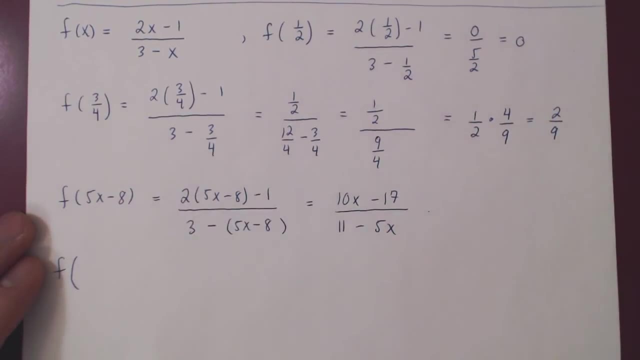 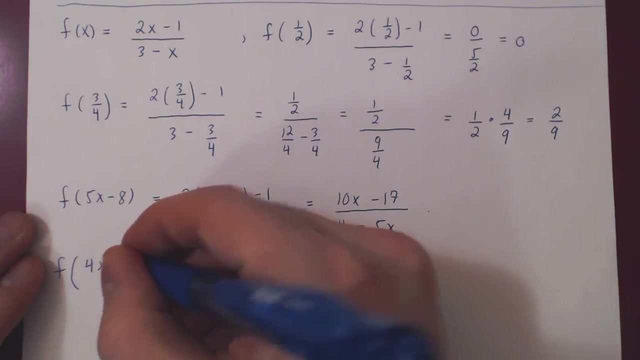 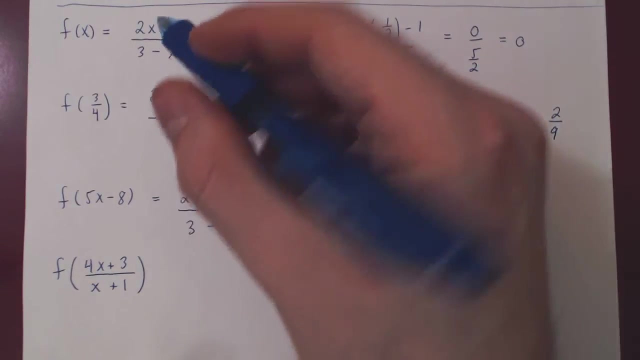 and our rational function of x, x by another rational function, and then we'll simplify it. So suppose we evaluate f of say 4x plus 3 over x plus 1.. So now we are replacing everywhere in the expression x by 4x plus 3 over x plus 1.. 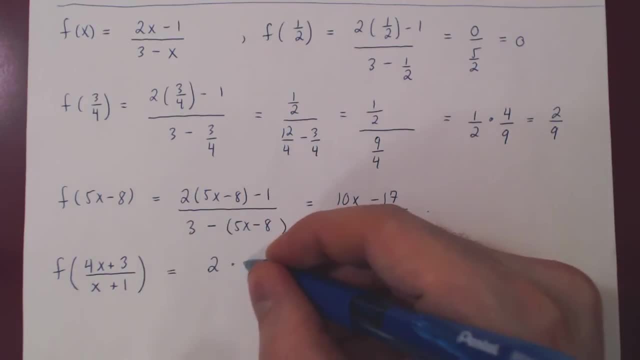 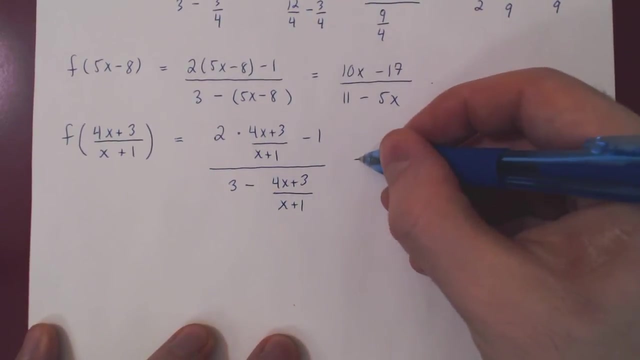 So we get 2 times this fraction minus 1, over 3, minus the entire fraction, Of course. now this looks rather silly. let's simplify it as a single fraction. Let's multiply our numerator by 2, which will give us 8x plus 6 over x plus 1.. 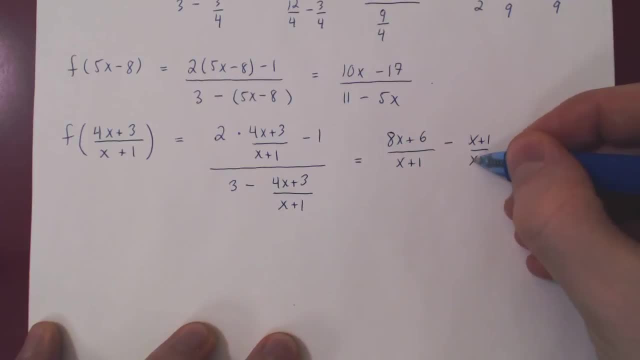 1, of course, is x plus 1 over, x plus 1, over. well, to simplify, we need this to be an over x plus 1, so multiply top and bottom by x plus 1.. And if you multiply it out, 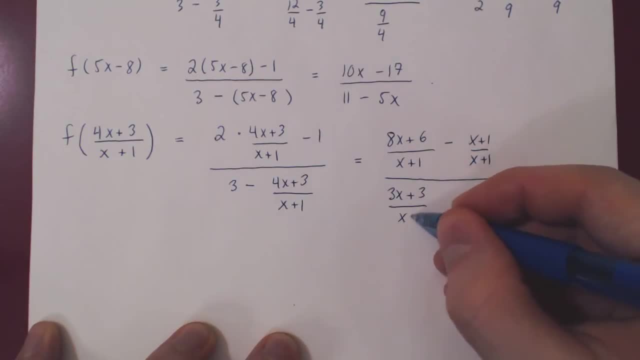 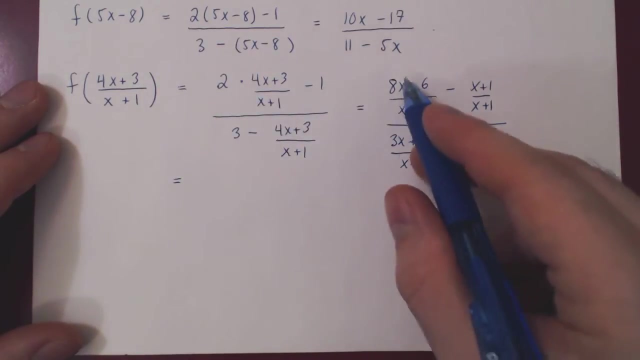 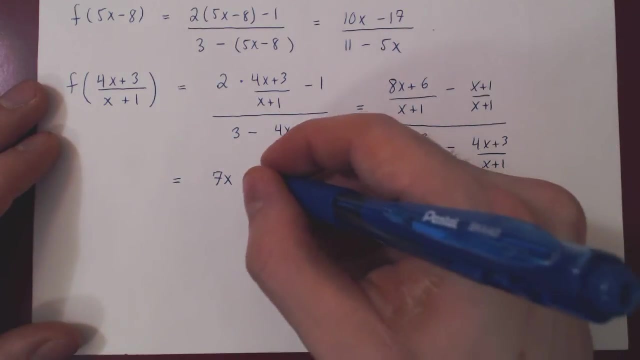 you'll have 3x plus 3 over x plus 1, minus the fraction 4x plus 3 over x plus 1.. Let's perform the two subtractions, So 8x minus x, 7x, 6 minus 1 plus 5, over x plus 1,. 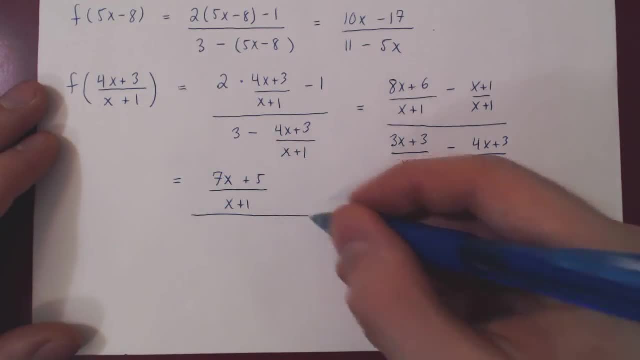 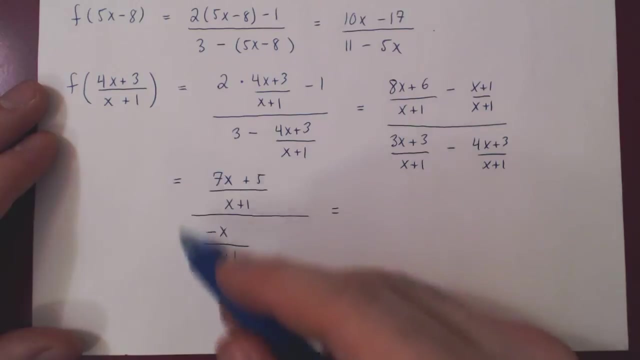 this is our numerator all over 3x minus 4x. so negative x 3 minus 3 is zero. So we get negative x over x plus 1.. And as before in the case of 1 half over 9 quarters. 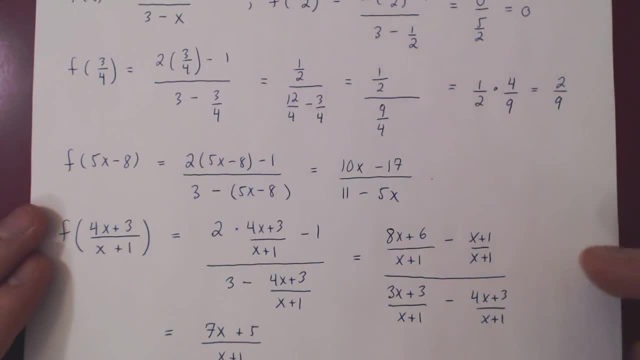 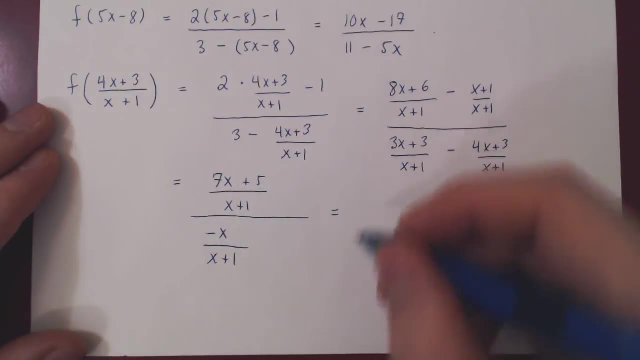 if we divide by a fraction, we multiply by its reciprocal. So let's do the same thing here. Our numerator is 7x plus 5 over x plus 1.. Instead of dividing by this fraction, we will multiply by the reciprocal. 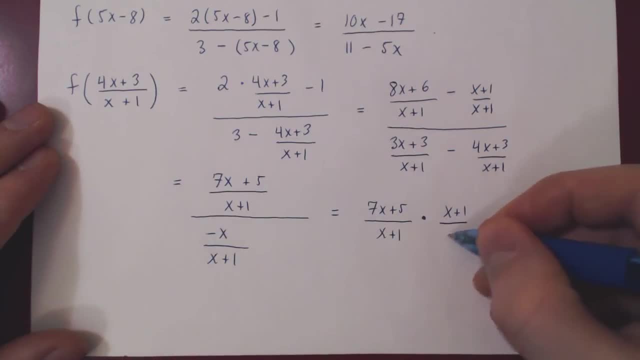 Therefore x plus 1 over negative x, Common multiple of x plus 1 on top and bottom we can cancel, And so we are left with 7x plus 5 over negative x. This looks kind of silly, so we'll move the negative as a constant multiple. 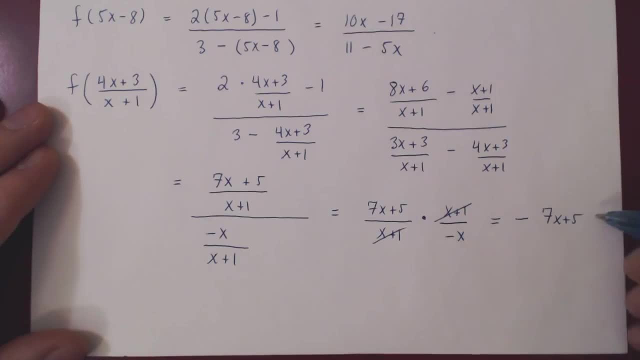 So negative of 7x plus 5 over x. If we wanted we could divide through And be careful here that the negative applies to the entire fraction. But if you divide through by x, both terms- 7x over x- is 7.. 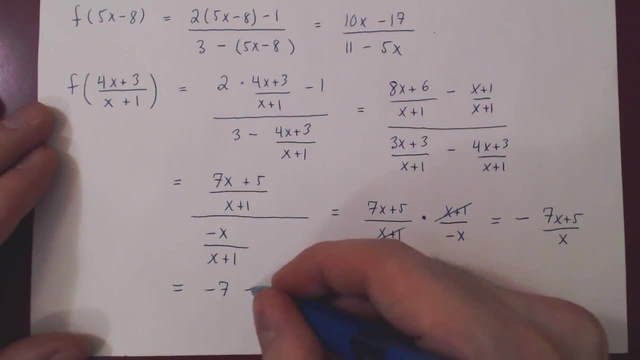 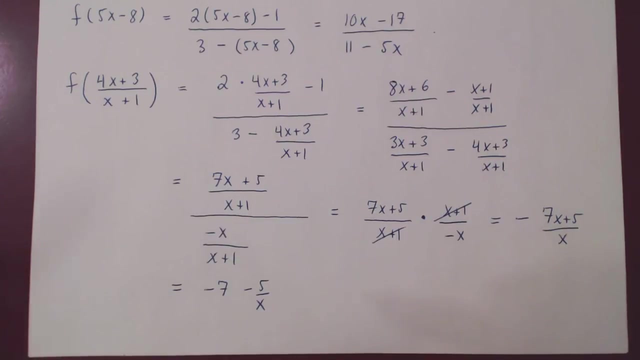 So it's negative 7. The negative: 5 over x, And this is now a matter of personal preferences, But either this or this one is fully simplified. So there you have it. So the idea is, if you have a function f of x equals some expression involving x. 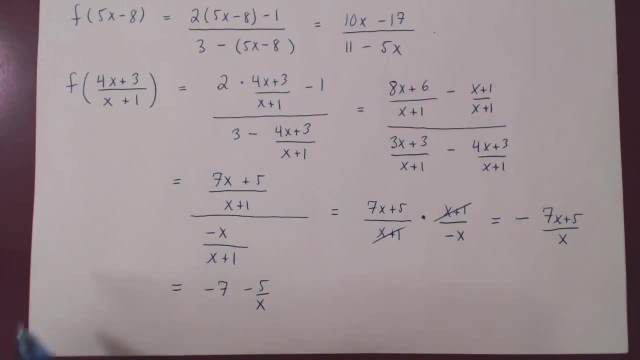 because x is a variable, you can replace the argument x by any other argument of your choice.